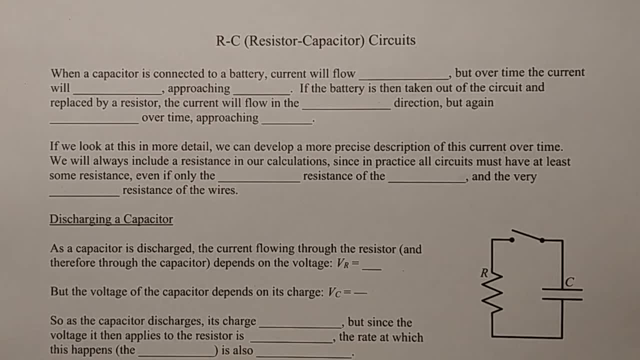 in something. Resistor capacitor circuits can be allowed to do this because it takes a certain amount of time for the capacitor to charge up to a certain amount, and so on. So when a capacitor is connected to a battery, current will flow initially. Initially it's easy because there's 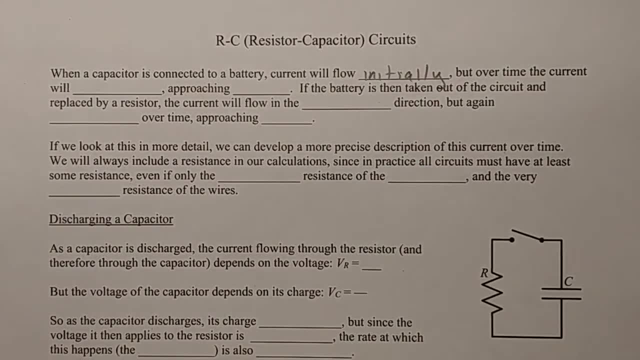 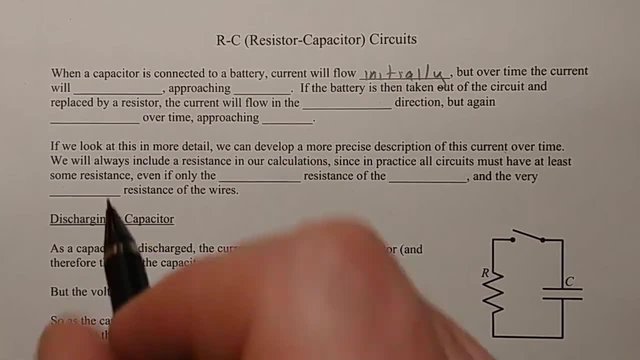 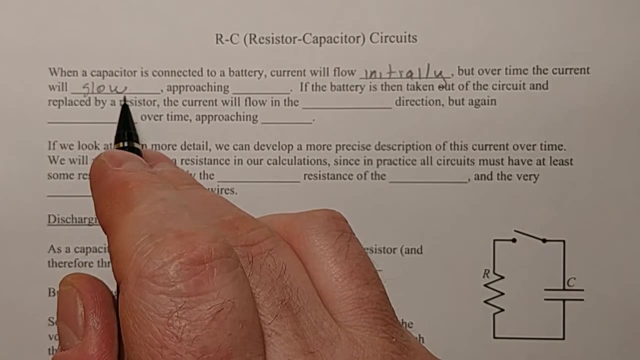 no charges on the capacitor. so charges can easily flow onto the capacitor and that's fine. But over time the current will slow down because as charges start to build up on the capacitor they push back on the other charges, making it harder for the charges to come on and eventually they will. 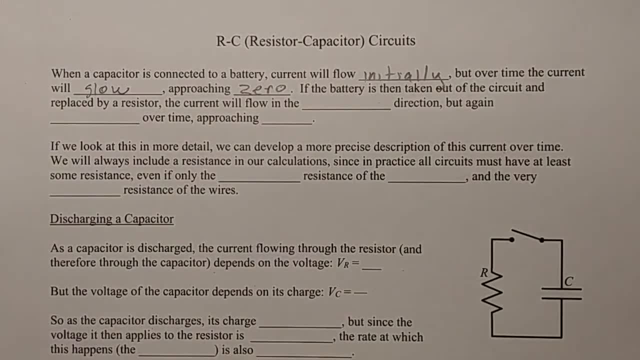 approach zero. If the battery, though, is then taken out of a circuit and replaced by a resistor, what can happen is we have all these positive charges on one plate and negative charges on the other, And so, if you connect the positive to the negative with the 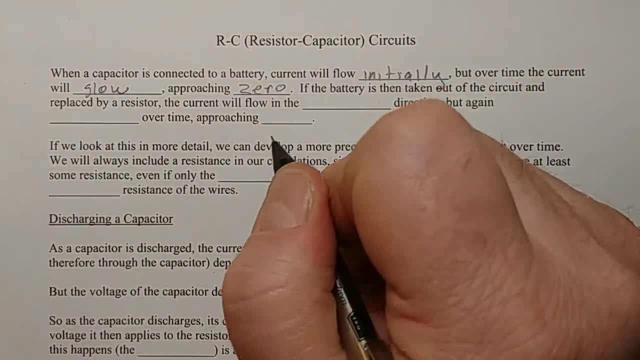 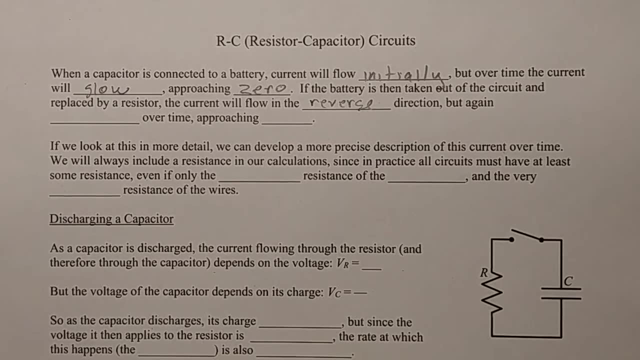 resistor. now what's going to happen is the current will flow in the reverse direction And initially there'll be lots of positives on the positive plate and lots of negatives on the negative plate. So the positive will be pulling each other, pushing each other, pushing positives. 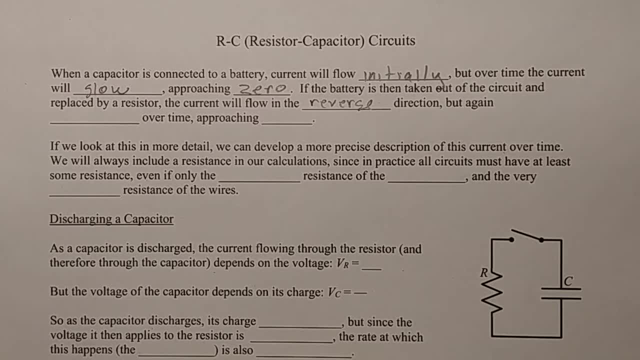 through the circuit down to the negative plate, through the resistor, But over time that will decrease. as the charges get less, the voltage will get less, so it won't be pushing as hard And um the it will take time, oh sorry, but again it will be decreasing over time. 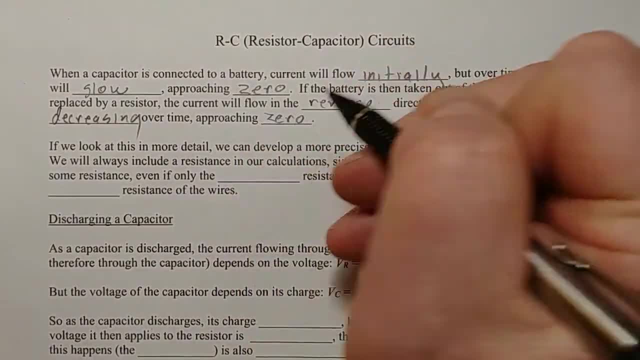 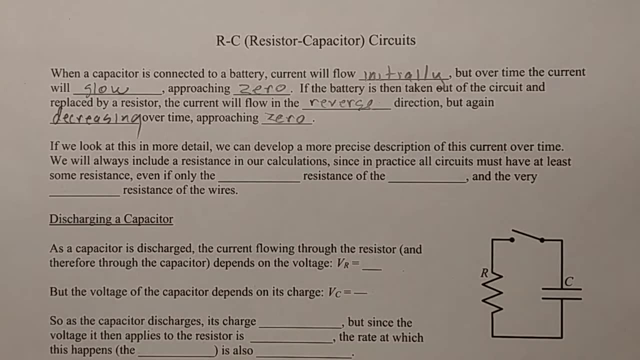 approaching zero once again. So this is basically what we can do. We can connect a capacitor to a battery and it charges up, And then we attach the capacitor to a resistor and now the charge charges, charge discharge. it discharges as the charges on the positive plate flow to the negative. 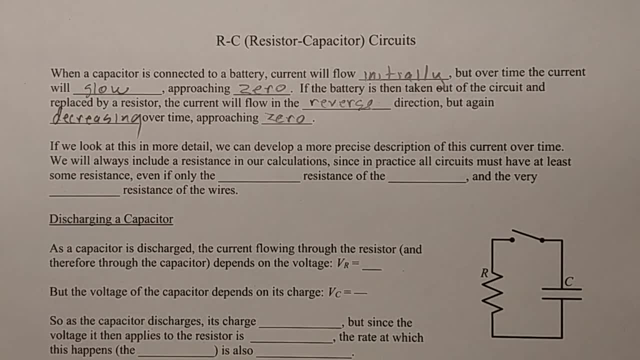 plate. Now, as we look in this more detail, what we're going to do is we're always going to include a resistance in our calculator. These are resistor capacitor circuit. There's no such thing as just a capacitor circuit. And the reason why there's no such thing as a capacitor circuit is because in 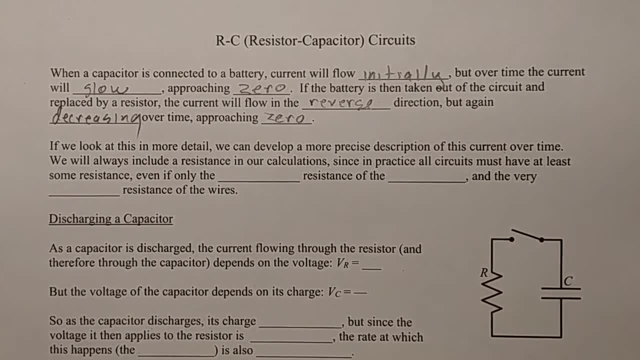 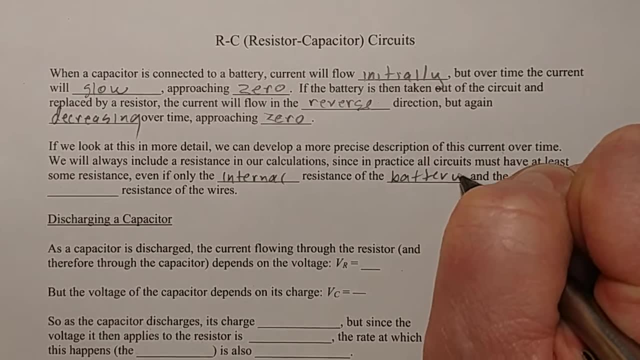 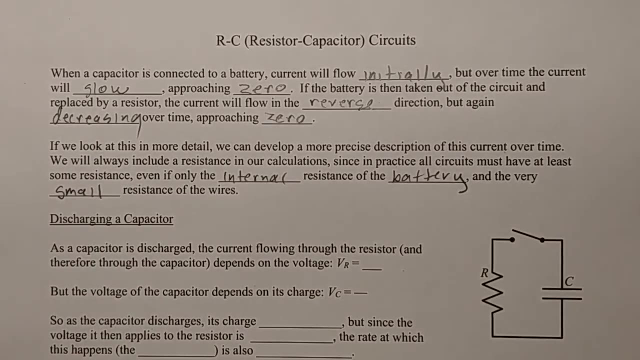 practice, all circuits must have at least some resistance, Even if it's only like the internal resistance of the battery, which we learned about before, and the very small resistance of the wires. and actually capacitors themselves have an equivalent resistance, because the capacitor has some parts inside where current has to flow through, And so there's some resistance in there. 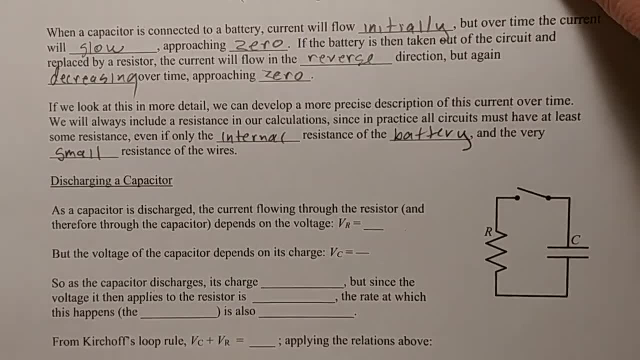 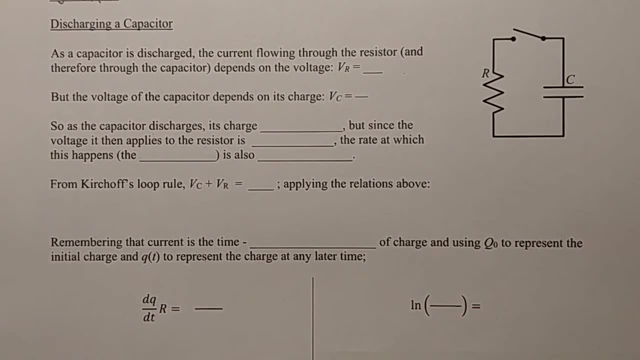 too. So there's always some resistance, but when we design circuits, we most often put a substantial amount of resistance besides that, But it just means that there's no point in doing that. I'm talking about a circuit without resistance, because it doesn't really exist. Okay, So here we. 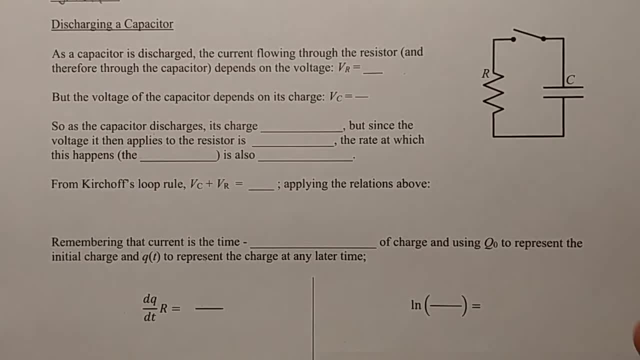 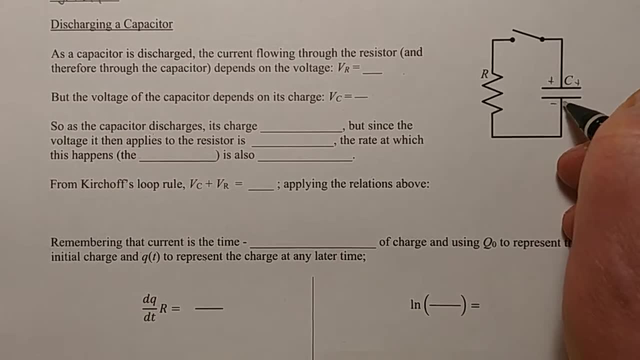 have. we'll start by discharging a capacitor, because that's sort of the easiest thing is. all we have is a capacitor and a resistor, And the capacitor starts off with a bunch of charges, So like there's a positive charges on this side and negative charges on this side. So this capacitor- 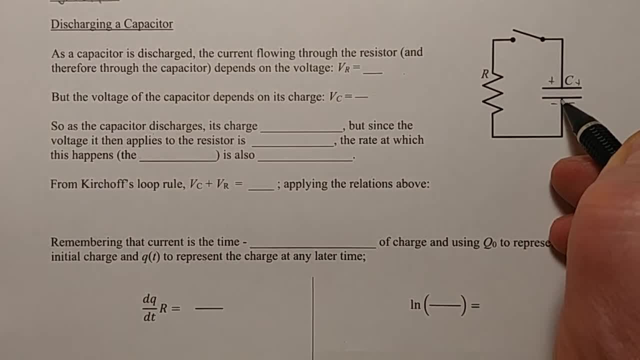 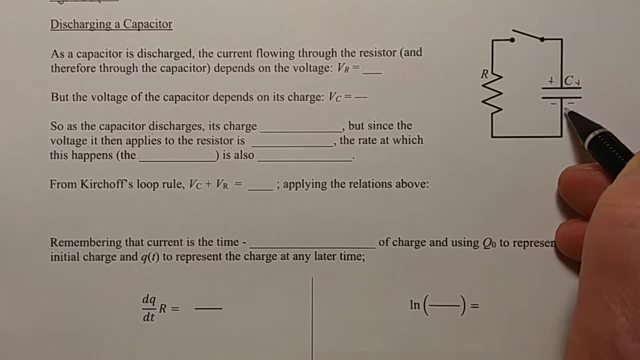 is charged up- There's positives here- They would like to go through the circuit and go to the negative side. Well, they can't do that right now because the switch is open. but if the switch closes they're going to be able to flow through that resistor and go to the negative. 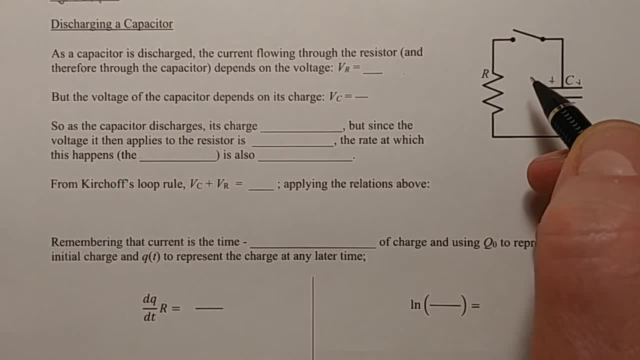 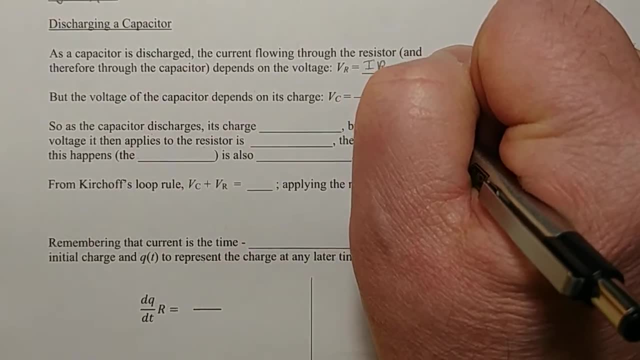 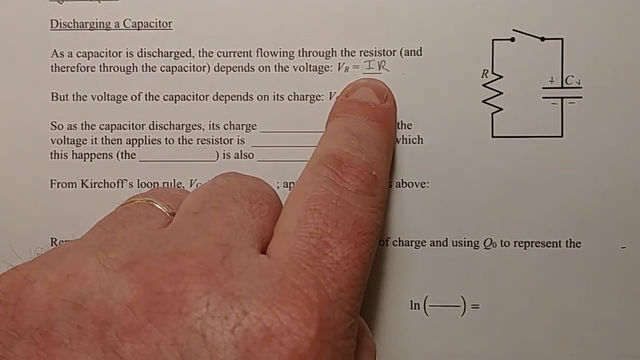 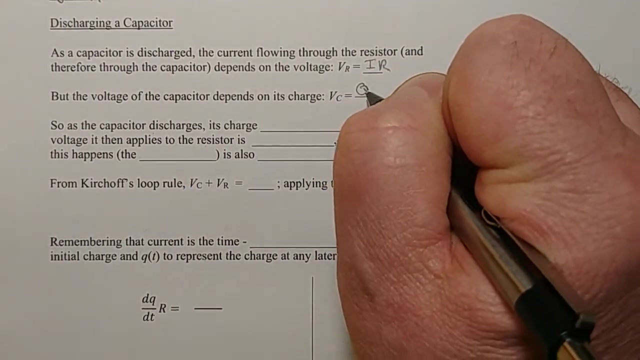 side Now as they're flowing. the current going through that resistor, we know, follows Ohm's law, which is V equals IR. So the bigger the voltage across the resistor, the bigger the current. but the voltage of the capacitor depends on its charge. You know that VC equals Q over the. 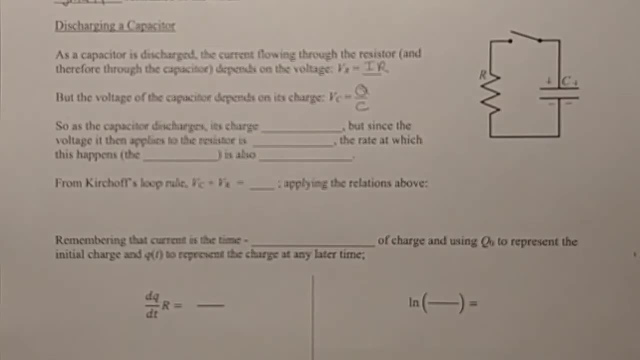 capacitance Q equals CV. So as the capacitor discharges, what happens? We start with a bunch of charges here, And so the charge is going to be flowing. and whatever charge is here means there's a certain voltage here which is pushing charges through the resistor. But as those charges flow through the resistor, 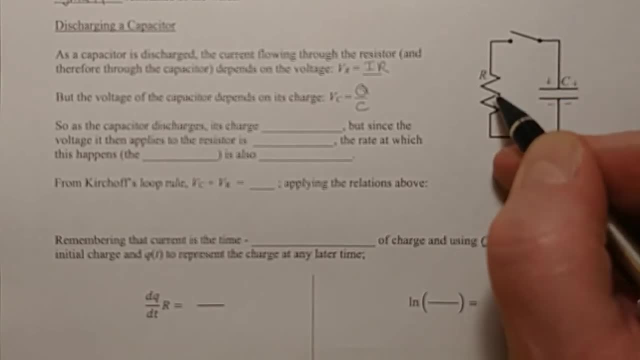 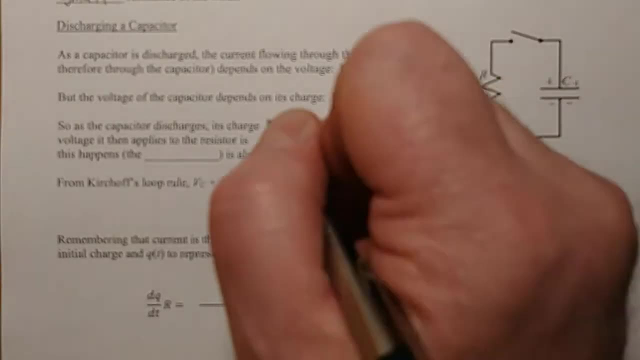 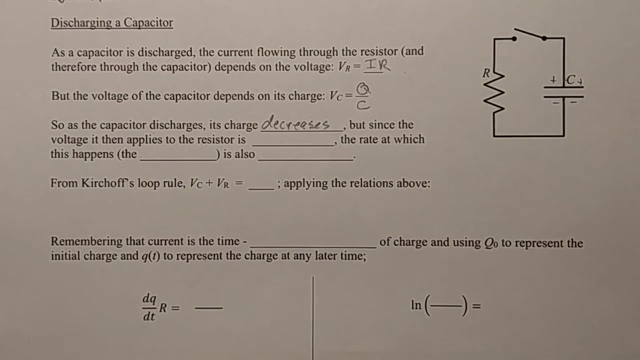 there's going to be fewer charges here, So they're not going to be pushing as hard, So not as much is going to be flowing, And so the flow is going to decrease. as the capacitor discharges, its charge decreases. But since the voltage then applies to, the resistor is lower with lower charge, it has lower voltage. 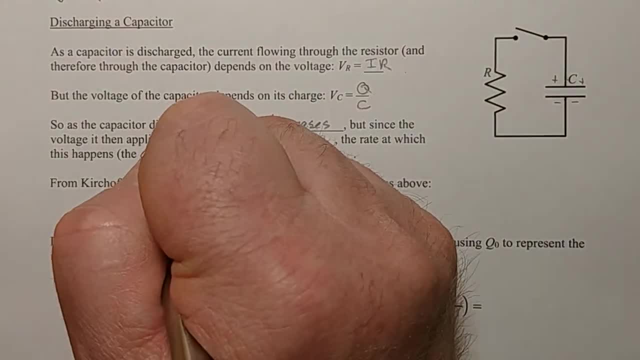 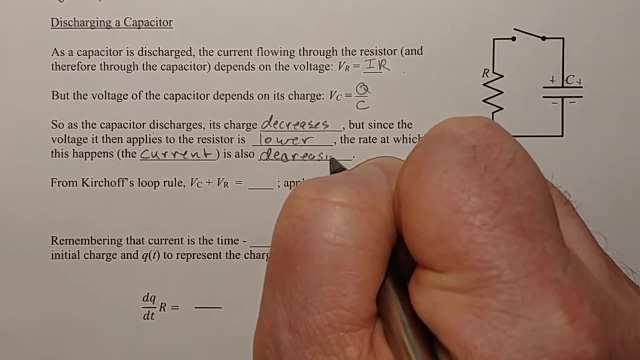 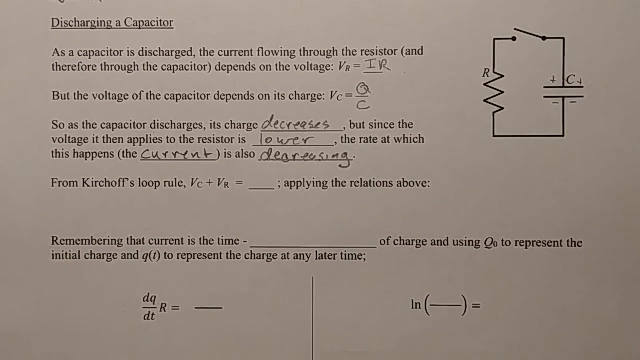 the rate at which this happens, the rate at which it's able to push charges through the resistor, the current is also decreasing. So a little bit of a, I suppose, a. what do you call that? Oh my goodness, I can't even think of the word right now. 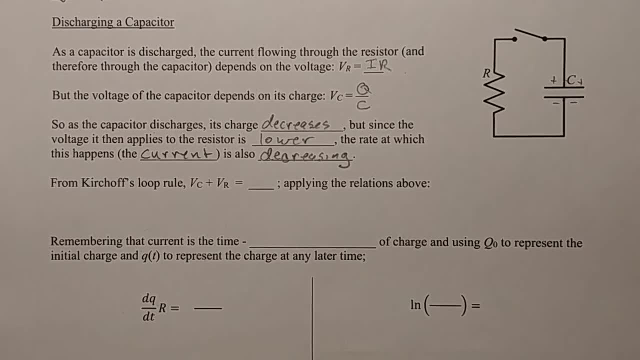 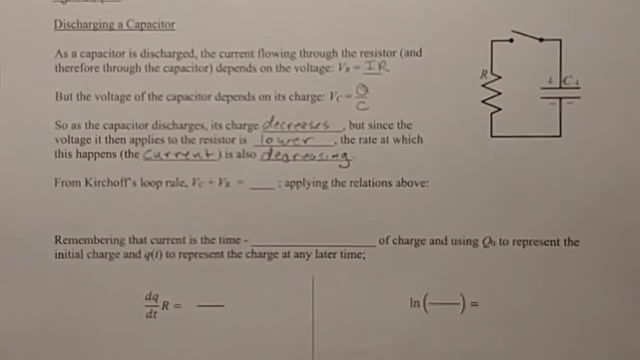 A spoiler, Spoiler alert, which isn't going to do any good because I'm going to say it anyway and you can't like. turn this off or you'll miss the rest of the video. This, by the way, says decreasing, is that in the process of our calculations down below, we're going to be: 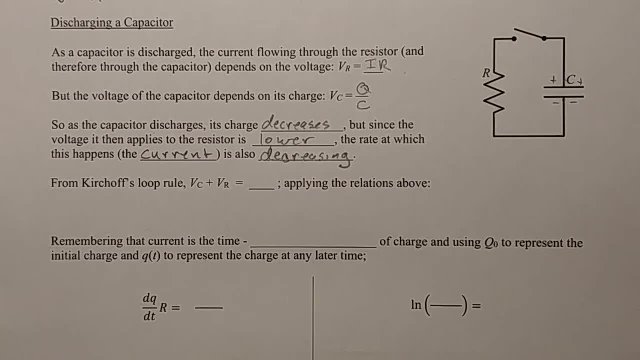 looking for a function that has to do with the fact that as it decreases, its rate of change also decreases, that its rate of change kind of has similar properties to the function itself. Gee, I wonder what the function that could be Okay. 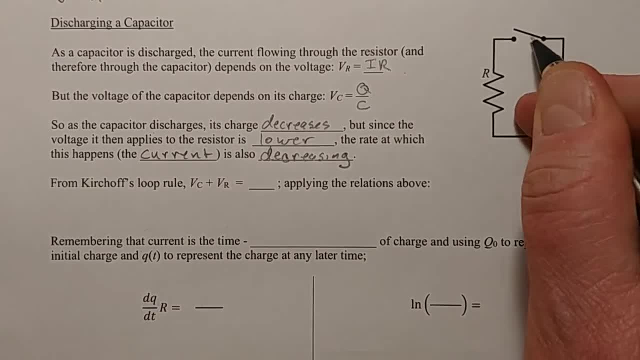 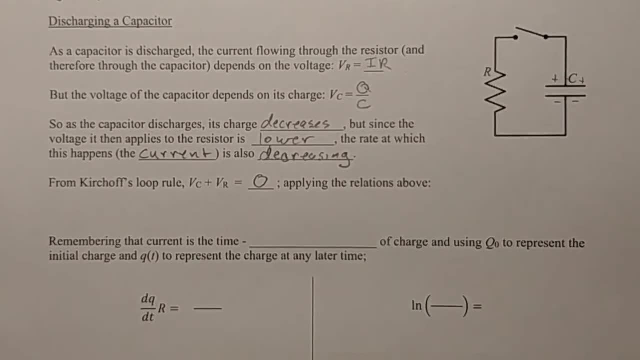 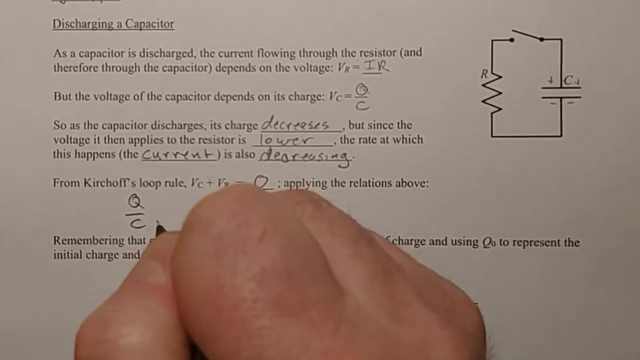 So from Kirchhoff's loop rule, we know that VC plus VR equals zero, And what I'm going to do is I'm going to apply the relations above. So what is VC? VC is Q over C, And what is VR? VR is IR and that is equal to zero. You might remember when we did Kirchhoff's? 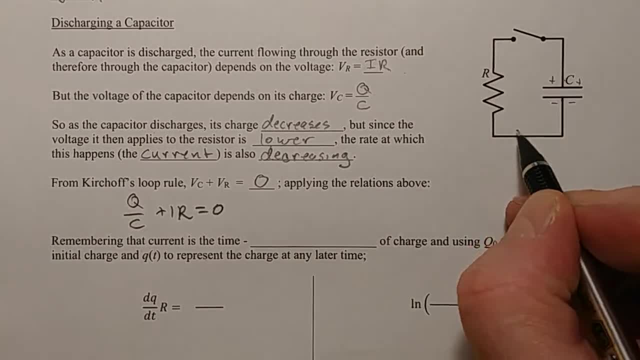 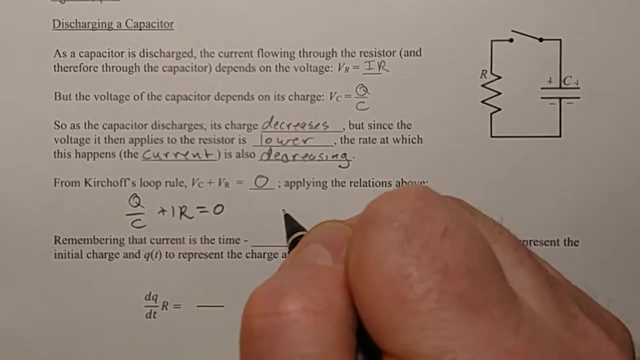 loops before we put a negative sign in front of VR because there was a voltage drop there. Kind of made sense then. but here it's not going to make sense because direction kind of matters in a different way And I'm just going to be fuzzy about that. but we're just going to leave. 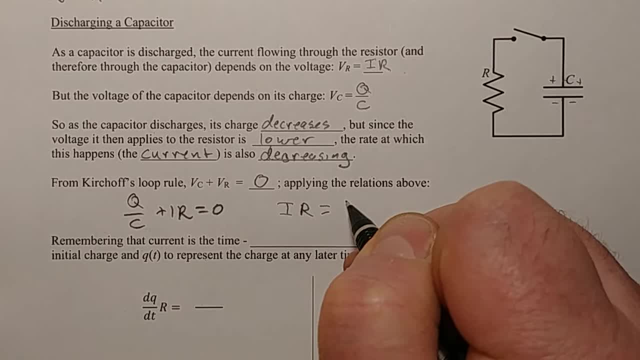 it like this And we're going to say: IR on this side equals negative Q over C. I don't know why I went from a capital Q to a small Q, but there you go, I did Okay. So the voltage drop and it. 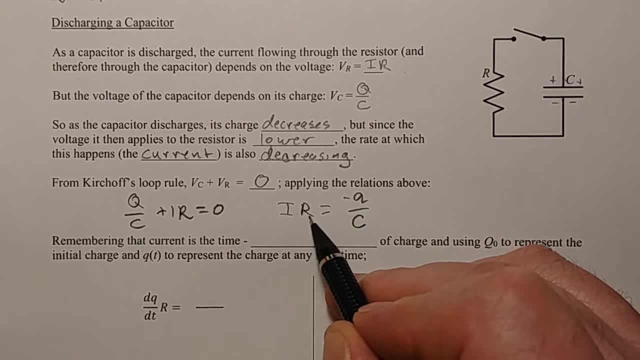 is a drop, the voltage drop- So we're going to say that Negative sign makes sense because it's a voltage drop- is equal to the negative of Q over C, Remembering that current is what is current. Current is the rate of change of charge. It is. 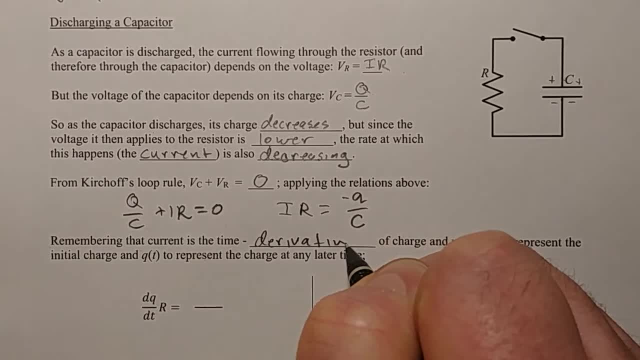 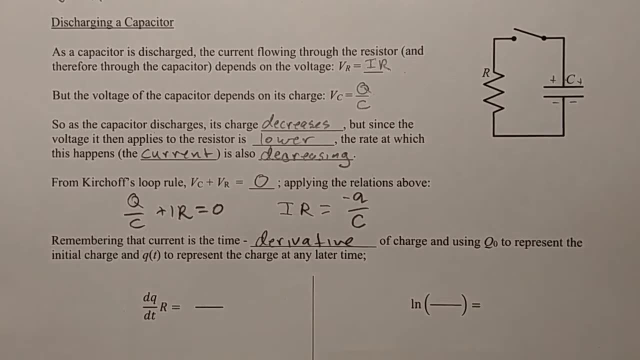 the time derivative of charge, And we're going to use Q naught. This starts with a certain amount Q naught. At the beginning it had a bunch of charge, capital Q naught- It represents the initial charge and later it has some other Q, which is a function of T. So what do we have here? 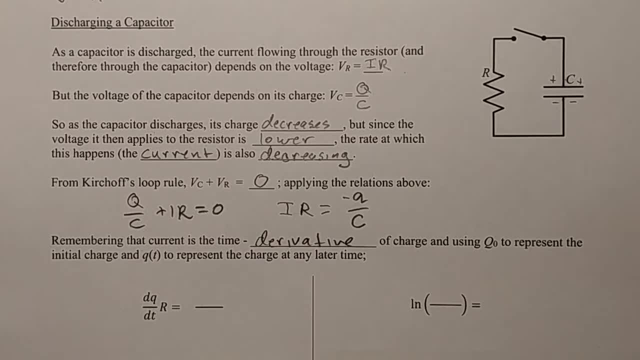 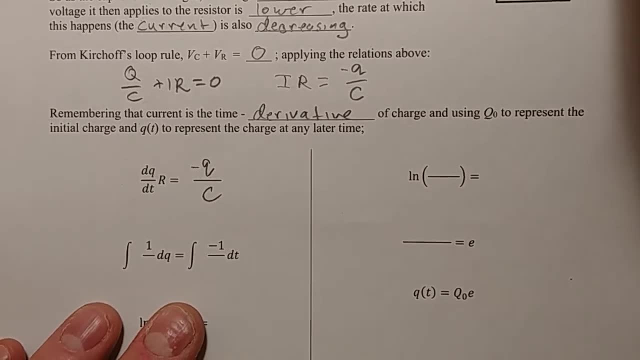 We have D DQ by DT times R. So IR equals negative Q over C. So let's see if we can have some fun with this. We're going to integrate this. The first thing we're going to do to integrate this is we're. 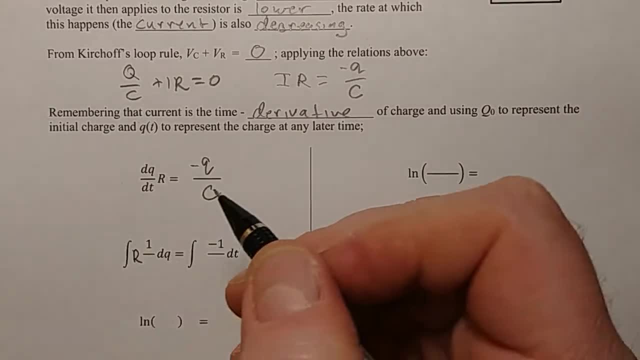 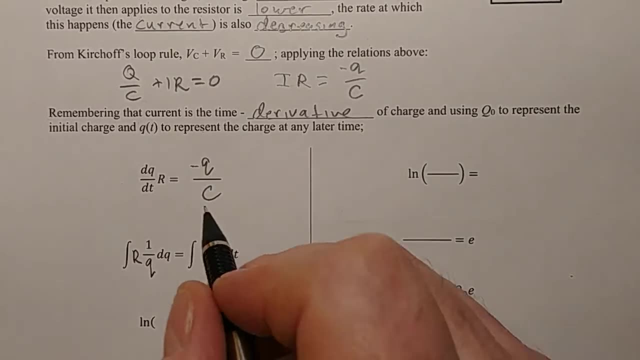 going to keep the R where it is, But what do we have here? We're going to put the Q down here because DQ is here, So let's put the Q over here with DQ, And then we'll just have negative one. 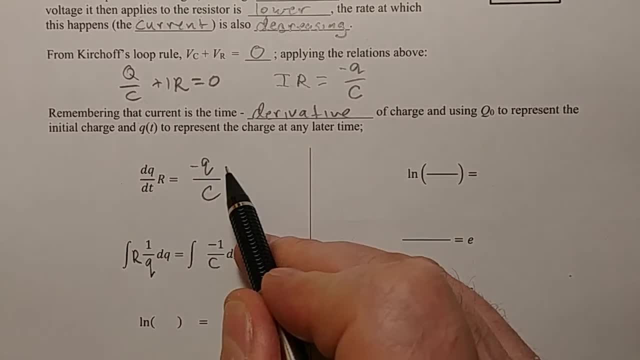 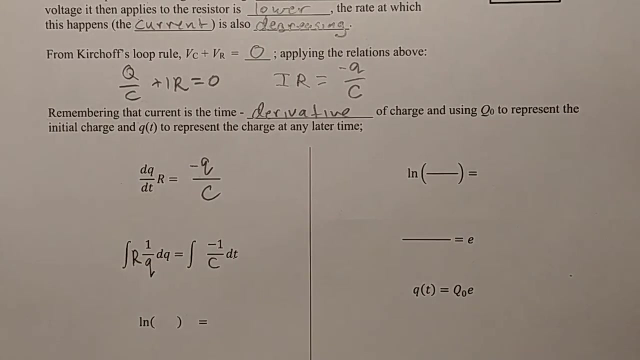 over C on this side. Is that right? I've put the T on the other side and multiply both sides by T And by DT, sorry, And now I've taken the integral of both sides, But these are going to be definite integrals. What are we doing So for the charge? we're taking the integral of charge from the. 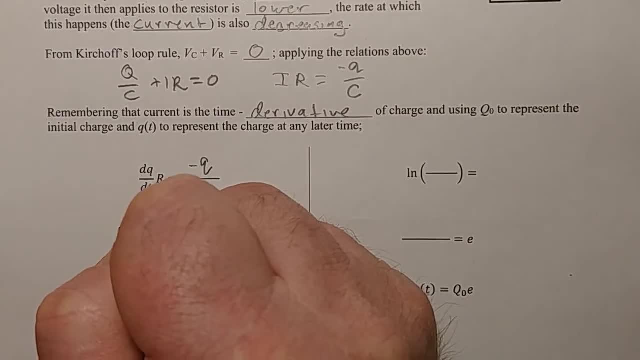 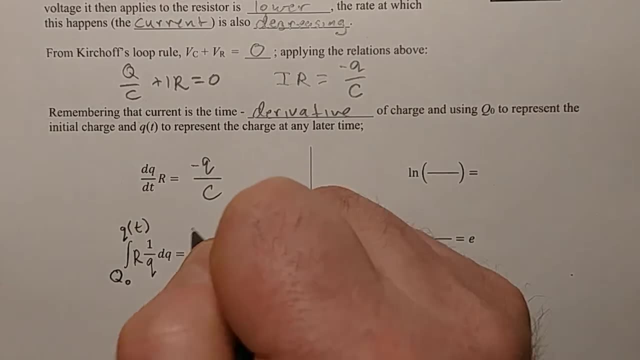 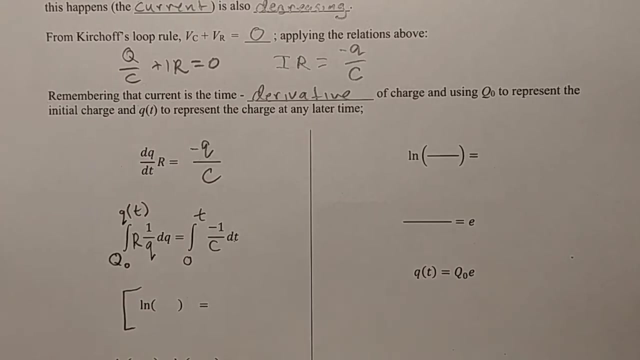 initial charge Q naught to some charge some later time And we're taking the integral with respect to time, from time zero, which is zero, to some later time T, So we have- Oh right, Isn't this interesting. What do we have here? We have R times, the ln. Oh yeah. 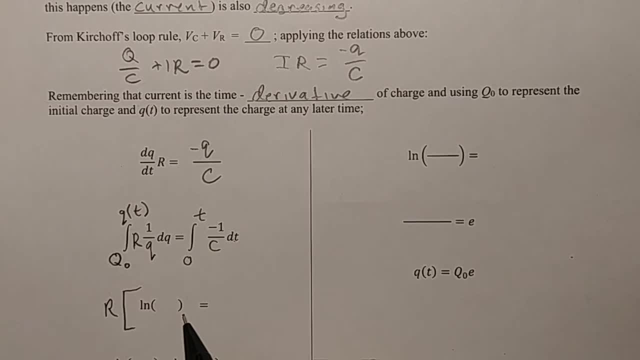 the integral of one over Q is the ln of Q. from Q naught to Q of T is equal to Well, the integral of this is just negative. Yeah, the integral is T. It's just T, It's just Yeah. 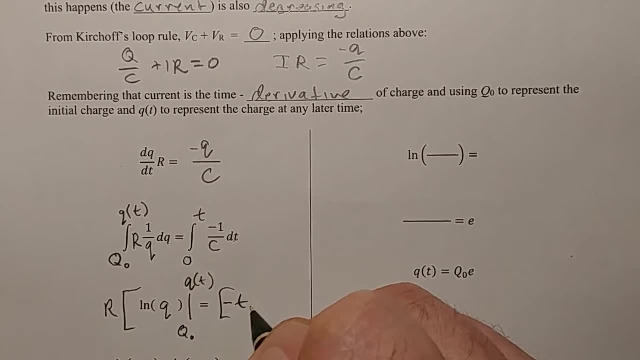 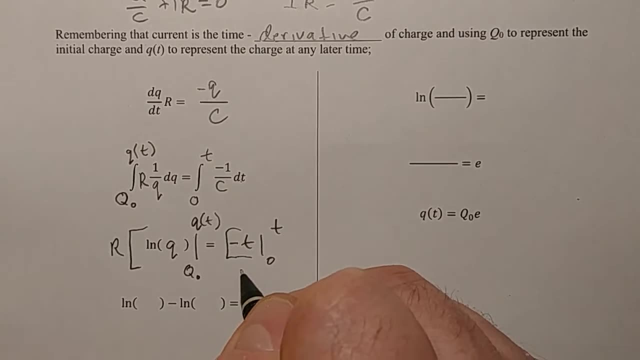 negative T, Negative T from zero to T. So what do we have here? We have the ln. Oh, wait a minute, There's a C under there. I forgot the C. I'm going to take the C and I'm going to put it down here. 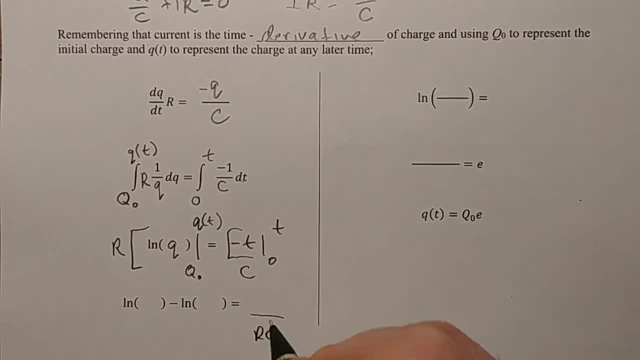 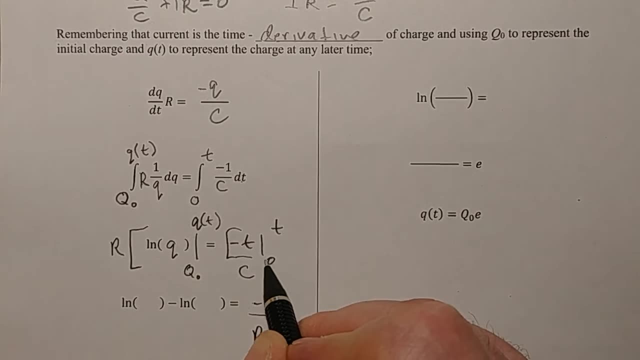 So it's RC And if I put the T in I get negative T over RC, And when I put a zero in there it's just zero. So put in the zero. I'm just going to. I hope you're okay with that. Okay, 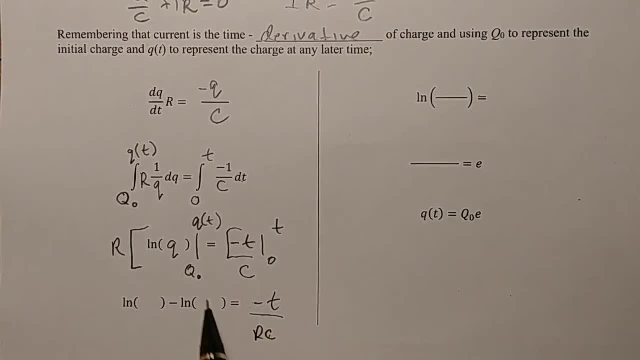 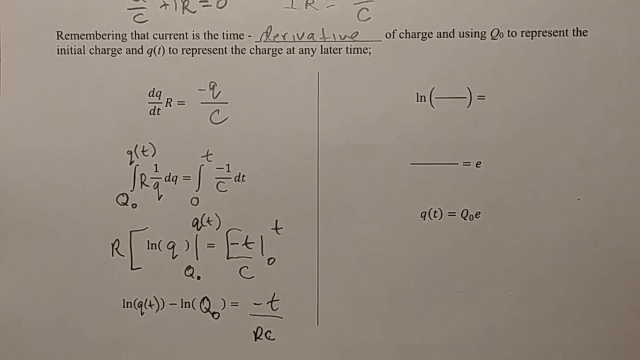 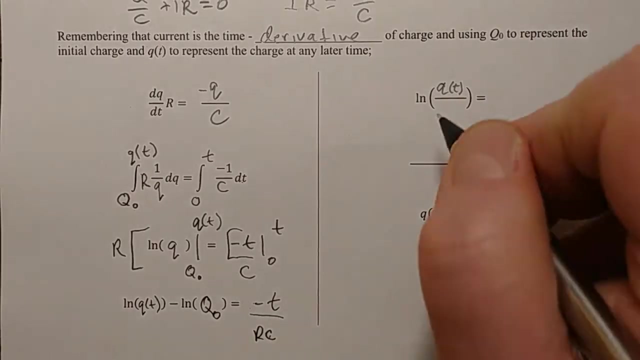 So what do we have here? Put it down there, That's good. Now I just have to institute ln of Q of T, Whoops, Minus the ln of Q naught. So what do we have? We have the ln of Q of T over the ln of Q naught. Sorry, what did I do? Oh? 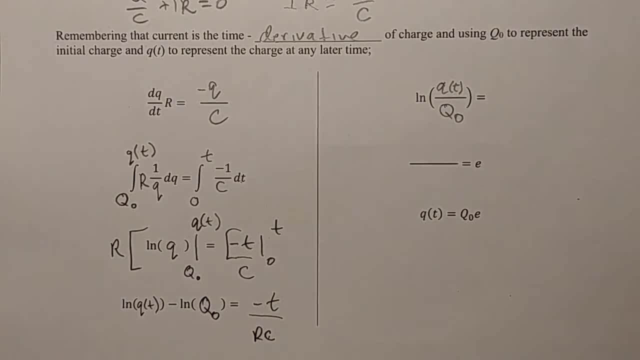 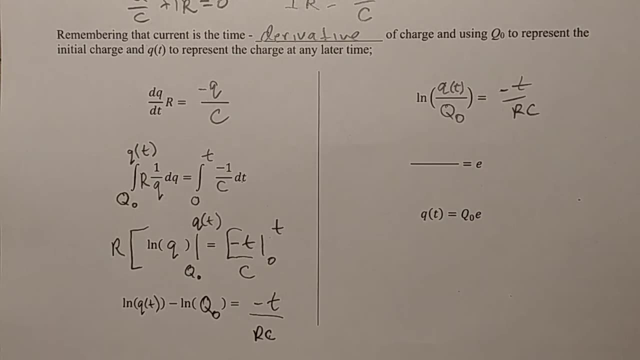 yeah, Subtract ln is like: take the quotient right. Yeah, That's cute, Equals negative T over RC, But I don't like the ln. So what I'm going to do with the ln is I'm going to raise both on the exponent E If I raise both sides on the exponent E. 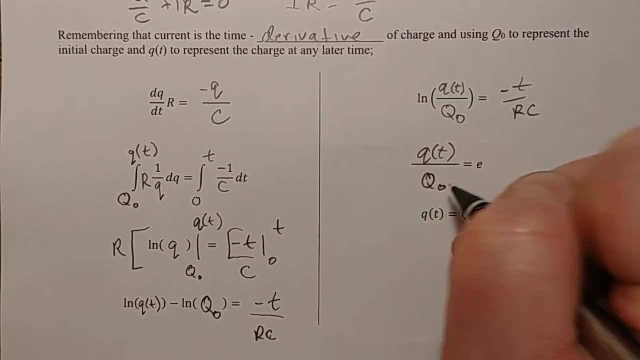 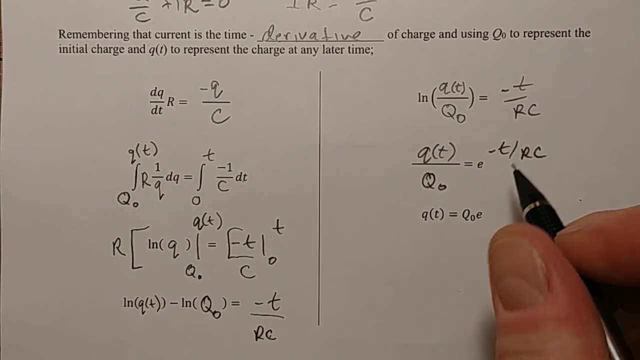 it gets rid of the ln and I just have Q of T over Q naught And this has been raised, So it's T over RC. So I'll take that Q naught over there and Q of T equals Q naught E to the negative T. 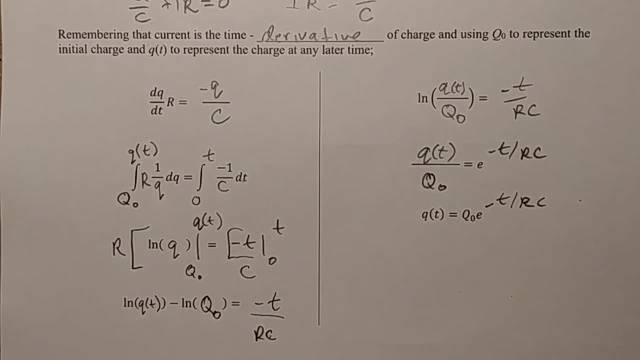 over RC. So that was a little bit of fun with calculus to show you. What we sort of intuitively understood from the beginning was that if the charge and the current are behaving in a circular manner, there must be some sort of exponential decay function involved. 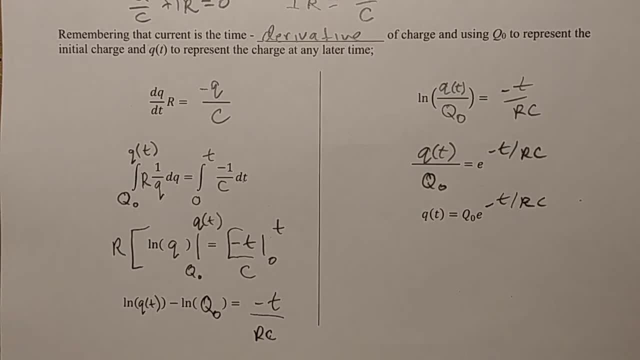 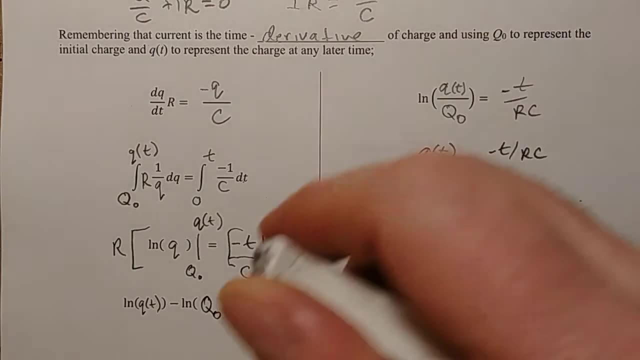 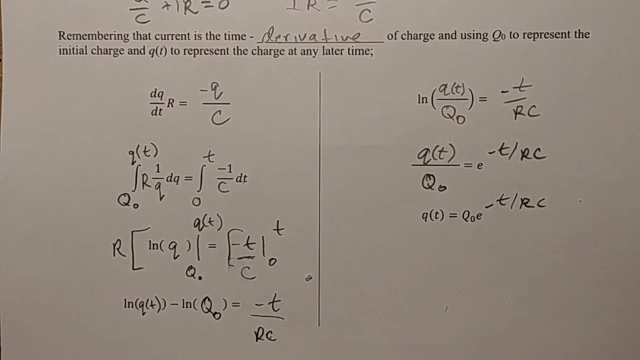 here because it is decaying over time, So it had to be exponential decay, hence the negative exponent. But there are some steps of wonderful calculus done a little bit messy. I don't know why I have that bracket there like so. But that's all beautiful And this is an equation that gives us 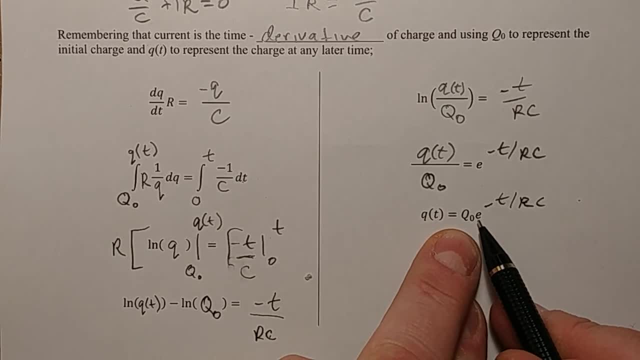 the charge over time On a capacitor which starts at Q naught and decays according to this equation.